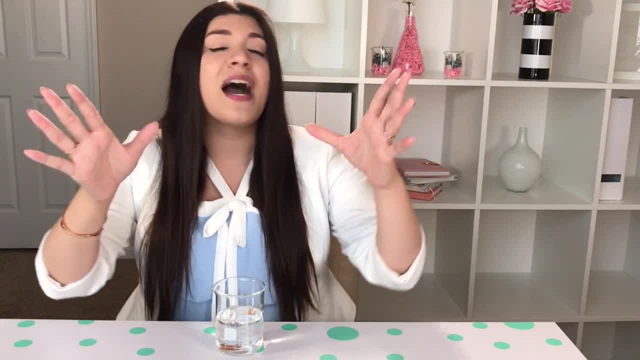 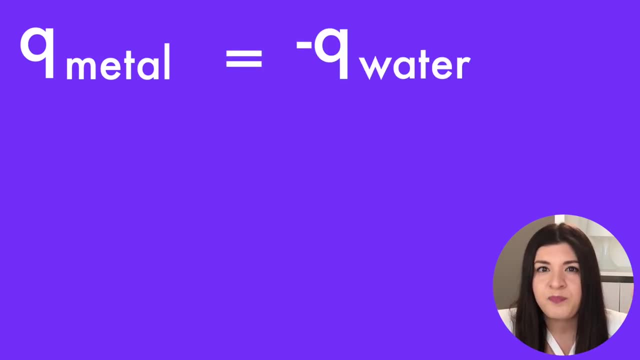 temperature. They're both going to have the same, All right. So that goes on to another formula where Q metal is equal to the negative Q of your water. Recall that Q is equal to MCAT and Q is your heat, which is equal to the mass times the specific heat capacity times your change in temperature. 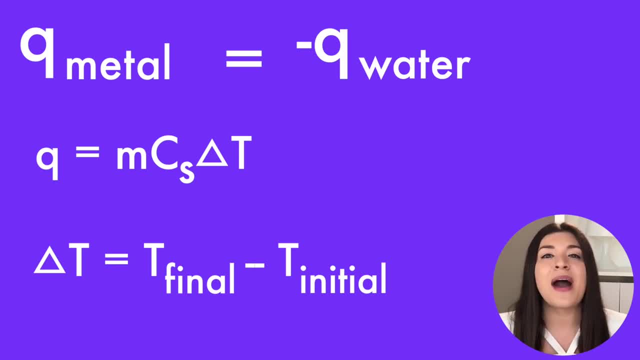 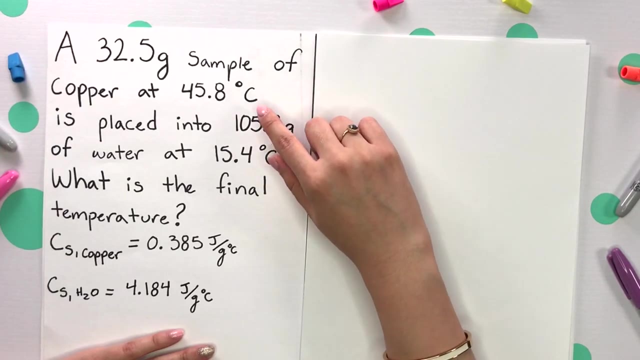 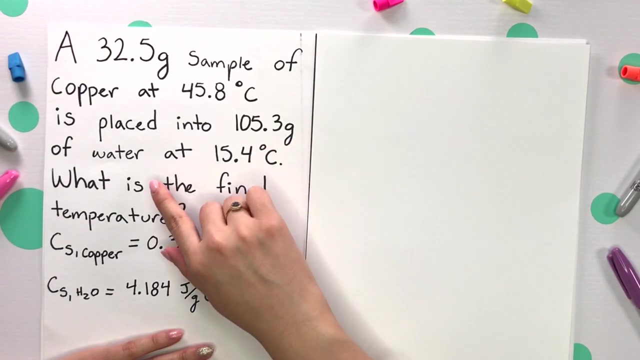 And your change in temperature is the final temperature minus your initial temperature. All right, So this formula, expanded, looks like this: Okay, Let's try one. A 32.5 gram sample of copper at 45.8 degrees Celsius is placed into 105.3 grams of water at 15.4 degrees Celsius. What is the final temperature? 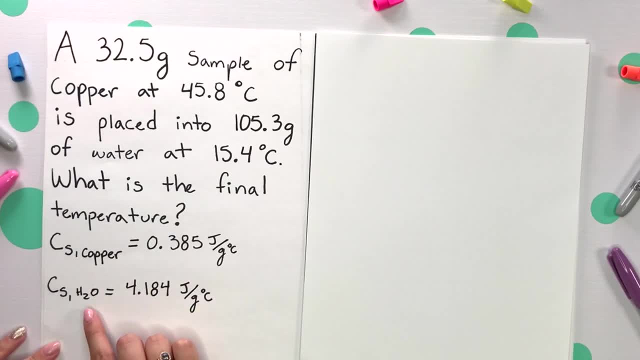 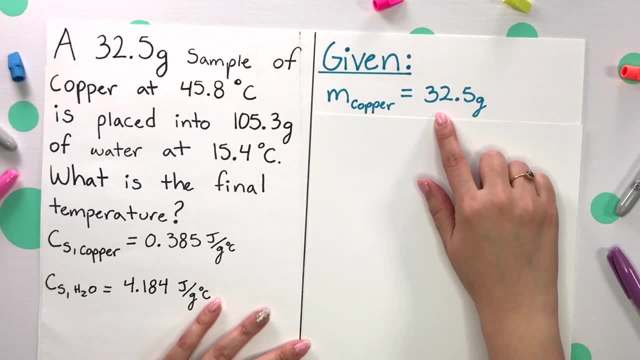 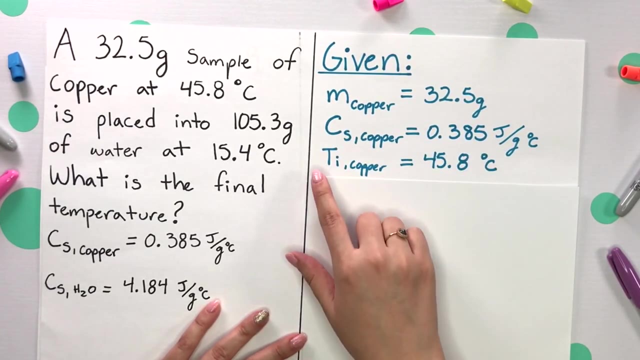 And you're given the specific heat capacities of copper and H2O. Let's identify our other givens. Your first given is the mass of copper, which is 32.5 grams. We're given our specific heat capacity of copper and your initial temperature of copper that 45.8 degrees Celsius. 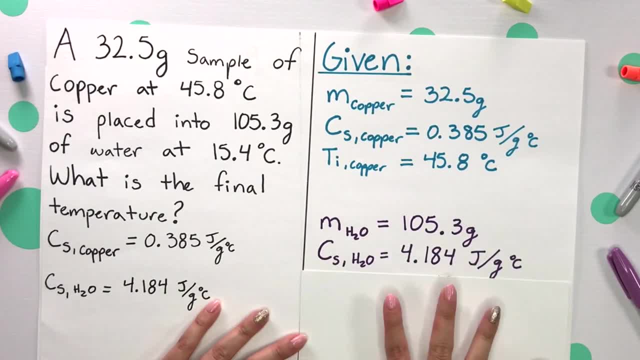 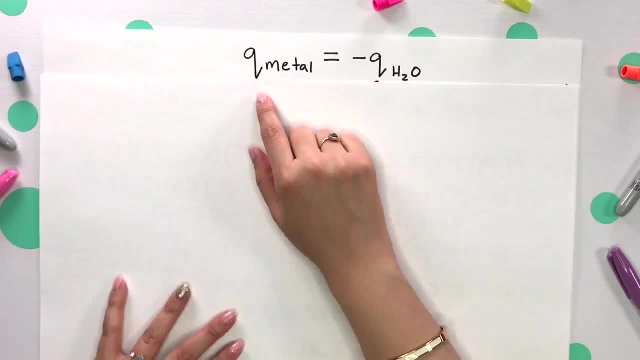 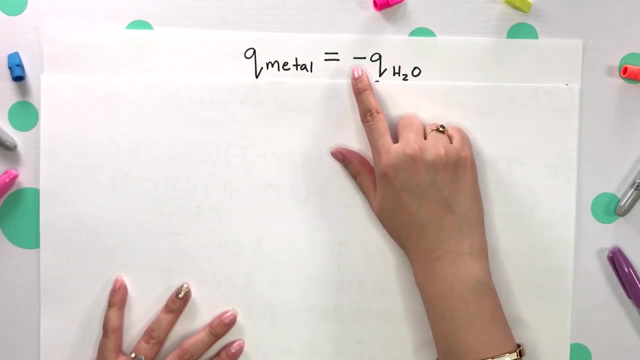 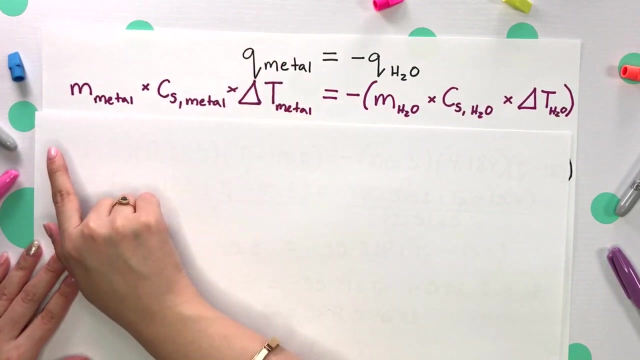 You're also given your mass of water, specific heat capacity of water and your initial temperature of water. The proper formula for this specific type of example is: our heat of our metal is equal to the negative heat of your water. Expanding this formula because you know that your heat equals MCAT, or the mass of our metal. 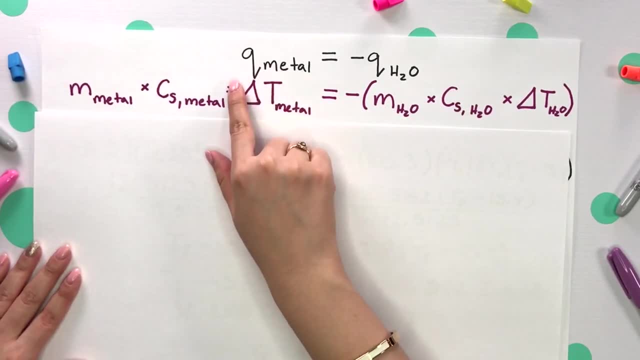 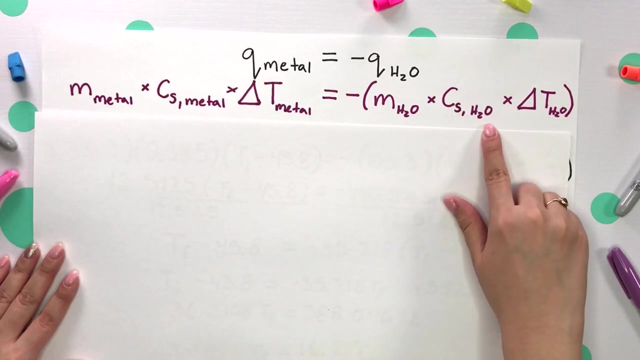 the specific heat capacity of our metal and our change in temperature. Remember, change in temperature just means your final temperature minus your initial temperature. We're going to set that equal to the negative portion of our mass, of our water, specific heat capacity of our water and the change in temperature of water. Plugging in all the